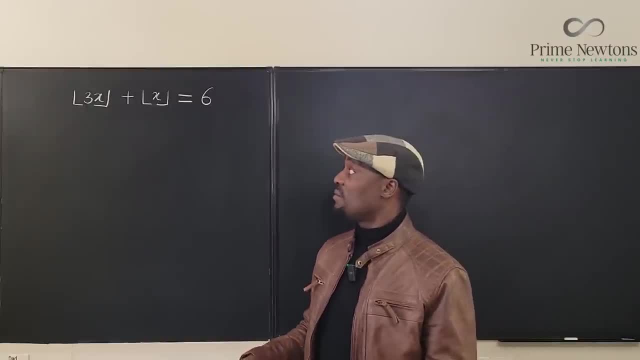 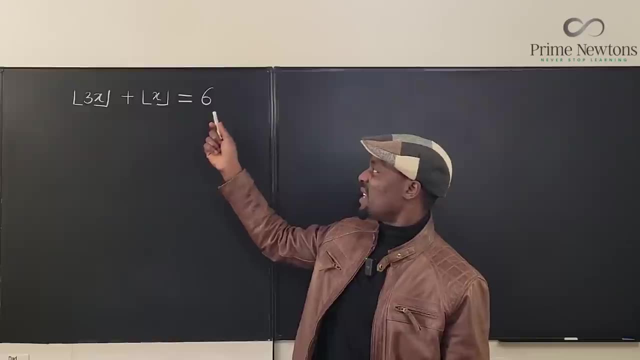 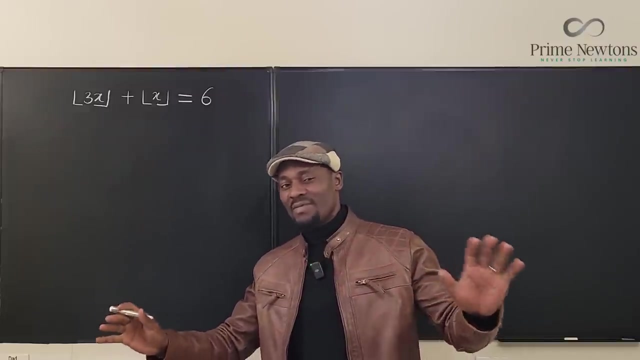 x is not an integer, because if it was an integer it would be either 1 or 2 or 3, and 3 times an integer plus x, another integer will be 6.. It doesn't look promising. So we know that x is not an integer. It's just so you can prepare your mind that our answer is not going to be an integer. 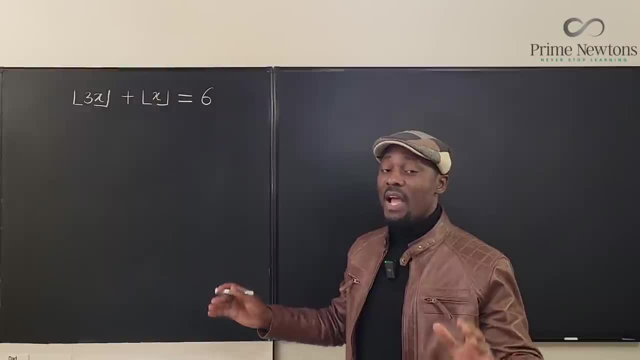 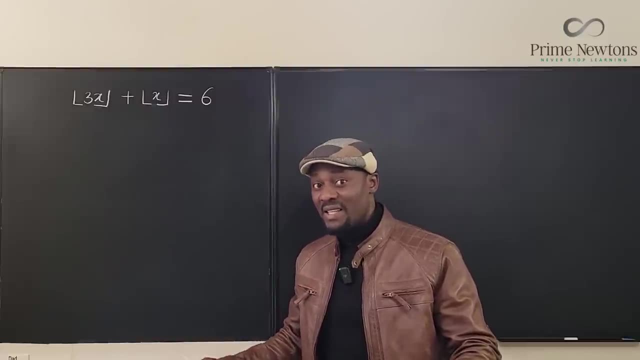 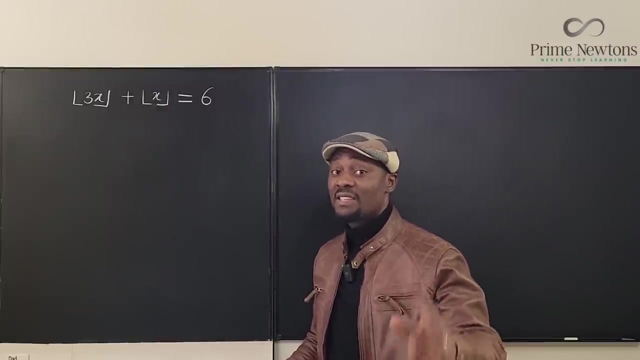 Okay now what does this mean? Let's go back again to the definition of a floor function. It's basically that there is an integer That is the floor of x, and that integer, if we call it k, has this property. 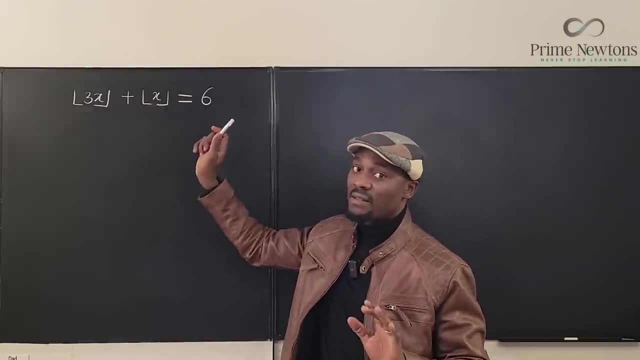 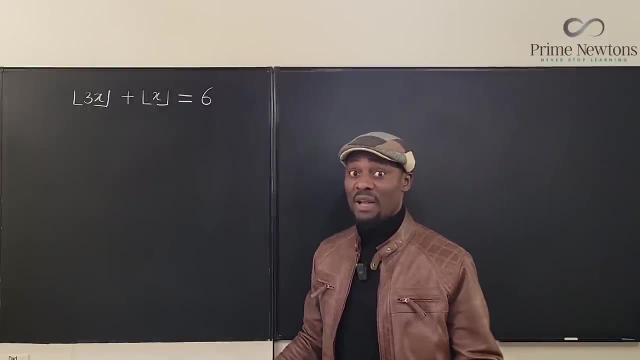 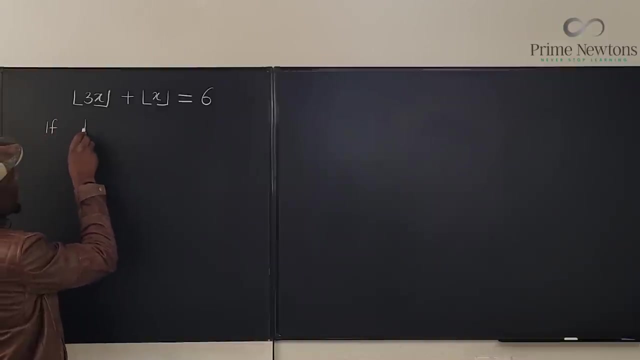 That k is either less than or equal to x. That's the meaning of floor. It's always under or they're at the same level. So we say that if k, if the floor of x, is equal to k, then 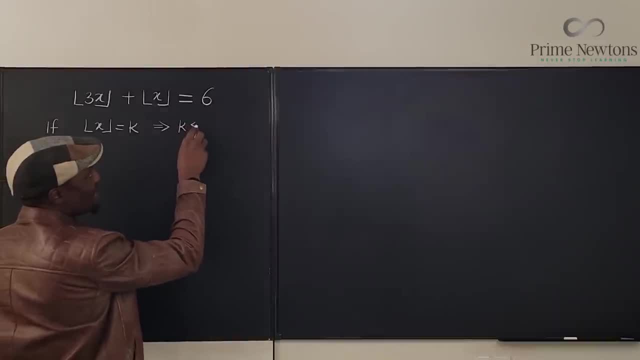 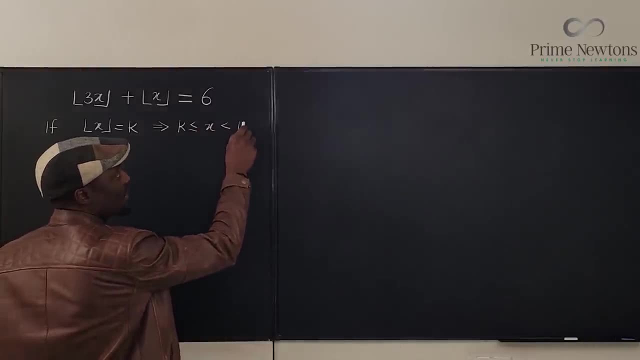 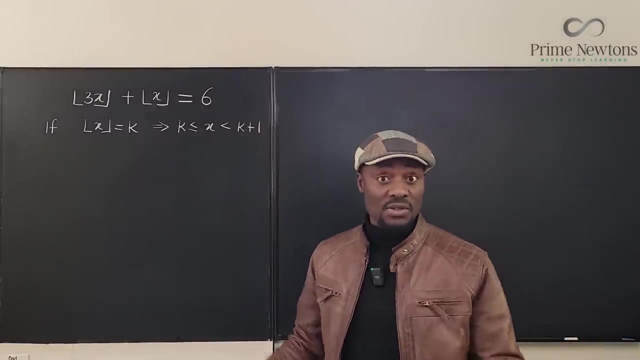 we know that k is less than or equal to x and x is less than the number that is next after k. We call it k plus 1.. This is very important in solving these floor and ceiling functions that we solve. So you know that if x is any number, 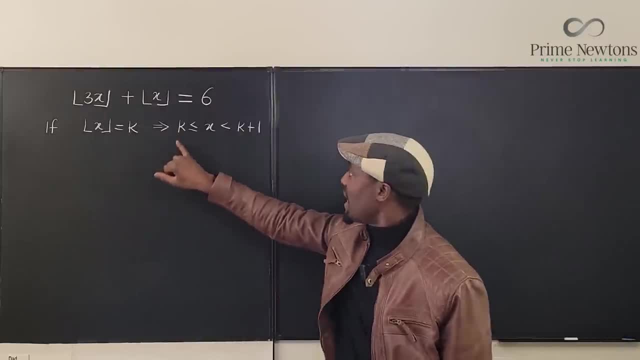 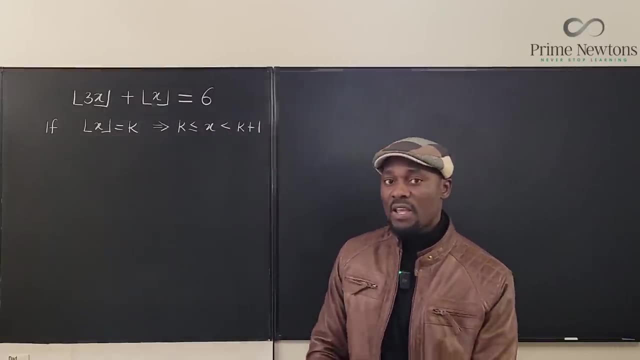 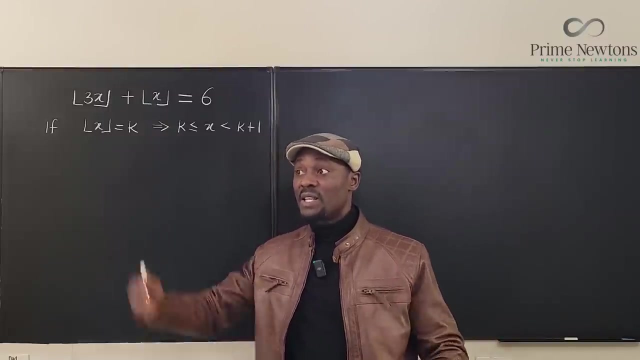 k is the floor of x means that k is less than or equal to x and that x is less than the number, the next integer. So if x is 1.2, then k must be 1, and we know that 1.2 is less than 2,, which is the next integer after k. 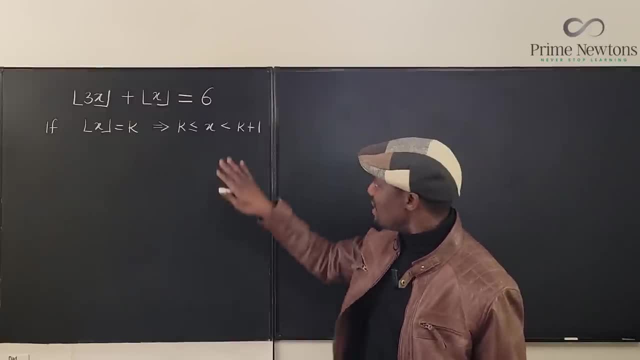 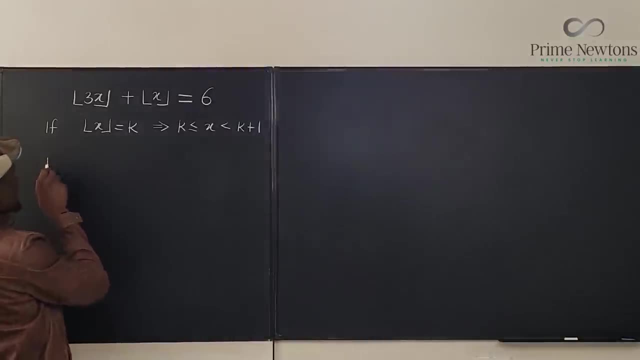 That's what you need. We need this, and then we need to do the same thing. for this. Let's do the same thing. Let's say: if t, if the floor of 3x is equal to t, then t is less than or equal to 3x. 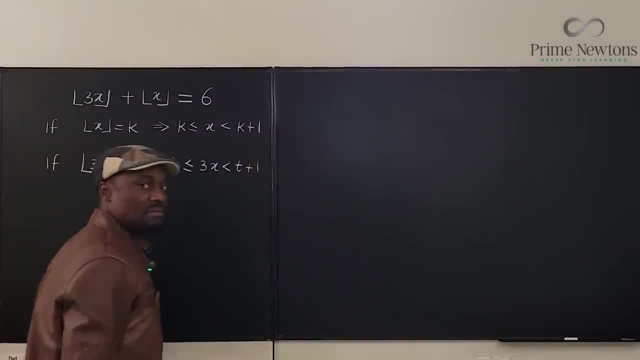 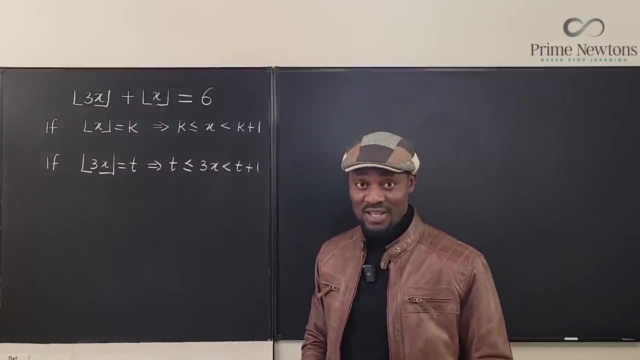 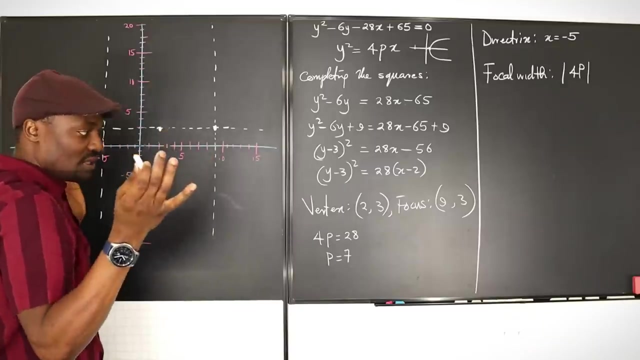 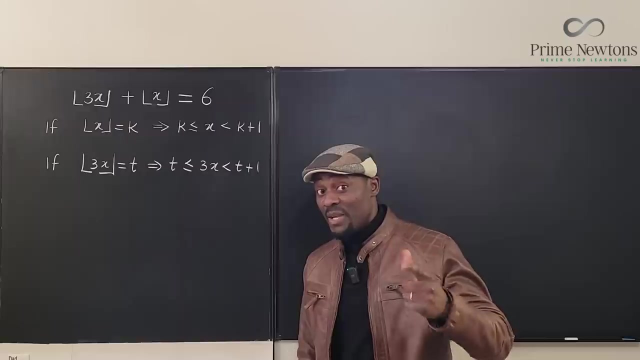 and 3x is less than t plus 1.. I promise you, these are the two things we need and we'll be done with this. Let's get into the video, Because our focus is supposed to be on x. I'm going to try to change this t. 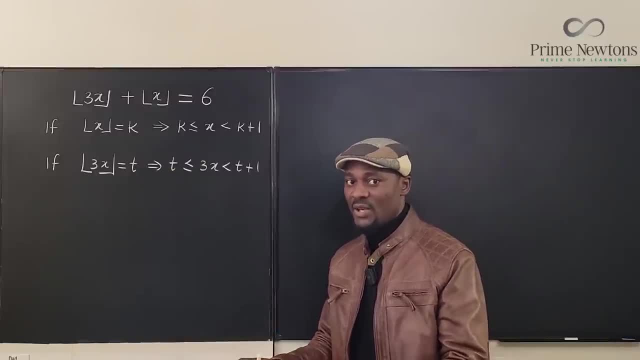 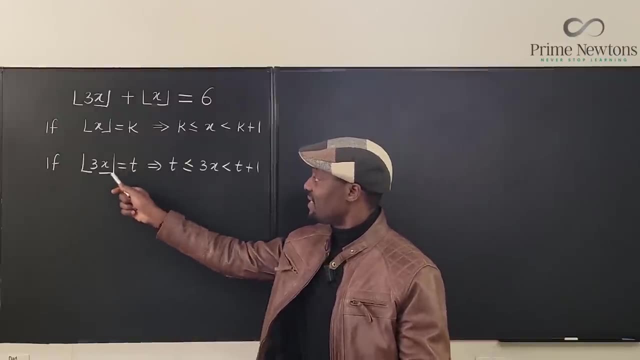 I don't want to have t in my calculation, I just want to have k. So we're going to think of it. What exactly is the best way to put these together? Well, remember that t is the floor of 3x. 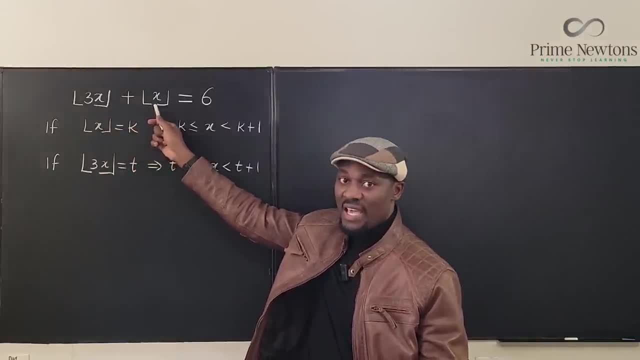 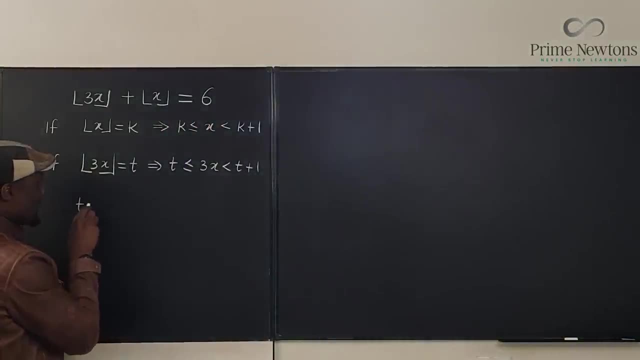 So we can replace this with t, replace this with k, and this is 6.. So we actually have an equation. We know that t, t plus k equals 6.. Which means that t equals 6 minus k. 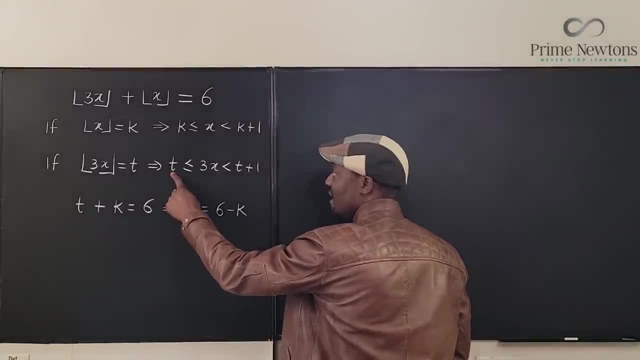 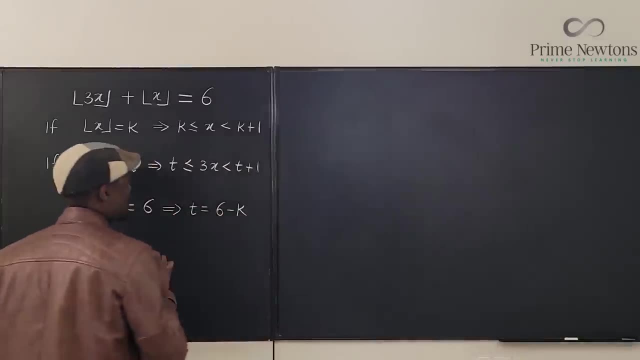 So what I'm going to do is, instead of writing t here and t here, I'm going to write 6 minus k, So we can have some nice equations to work with. So let's do that. So we're going to say that. 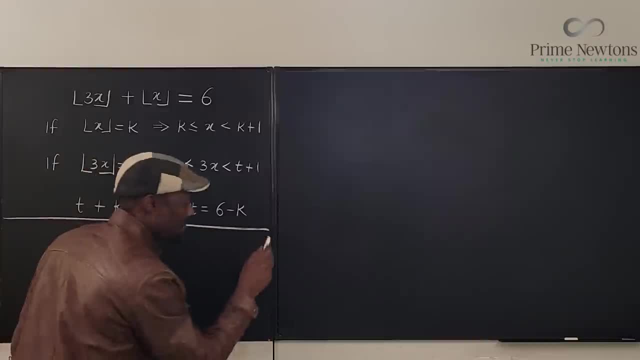 for the first equation. let's rule a line here. For the first equation. we have not equation inequality. We have k is less than, or equal to x less than k plus 1. This one does not have the equal to option. 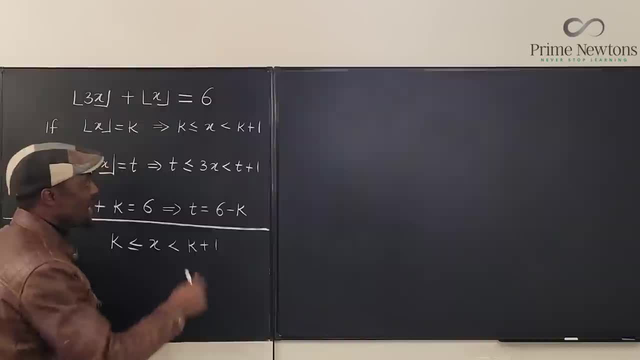 It cannot be equal. Okay, it has to be less than the ceiling. Now, in this case, we have t. Instead of writing t, I'm going to be writing 6 minus k. So I have: 6 minus k is less than or equal to 3x. 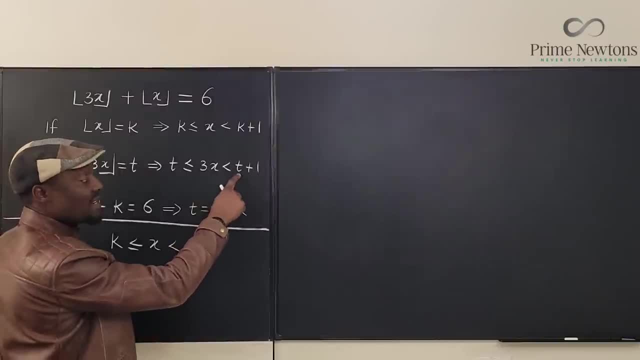 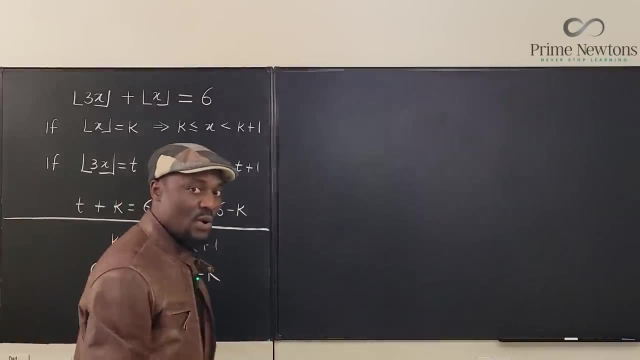 And it's less than. instead of writing t here, I'm going to write 6 minus k plus 1. which is gonna be seven minus K. These are the two inequalities that I need. Now let's start thinking precisely, okay. 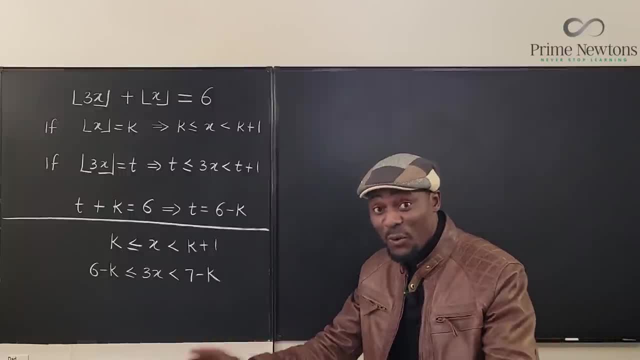 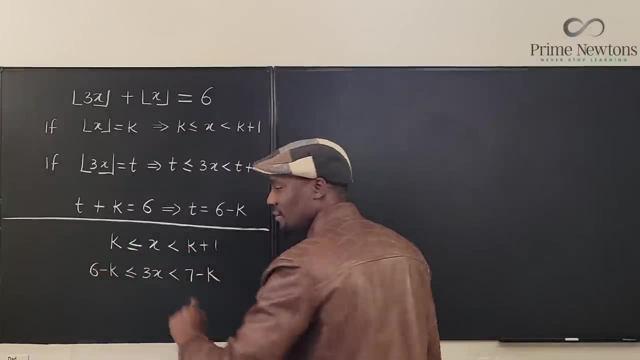 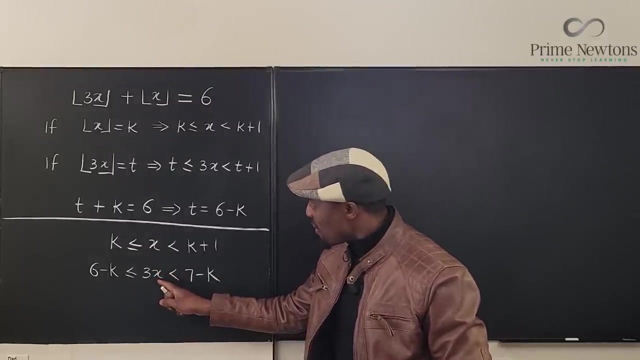 Think very well, because we're gonna use these two only to solve the entire problem. Let's start with this. Oh wait, can we make this and this look alike? Yes, why don't we create an X here? We can easily do that. 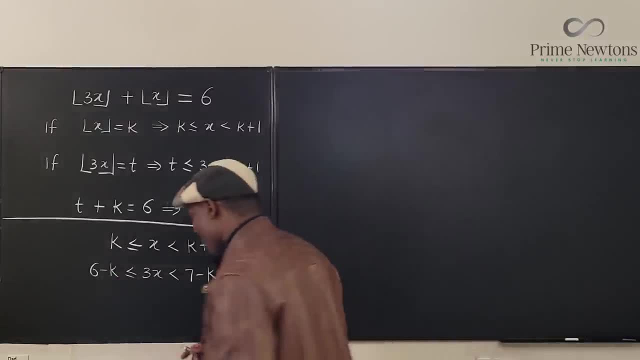 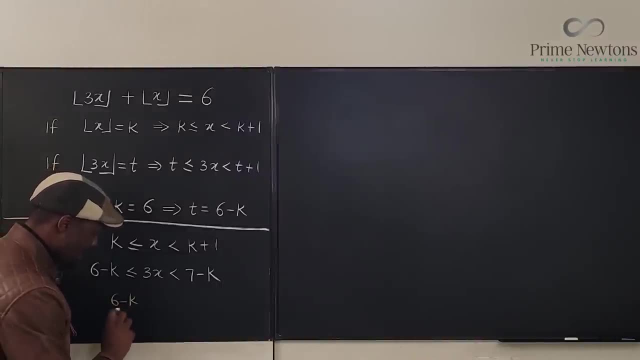 by dividing each of these sections by three. Let's do that. So if we divide each of these sections by three, we're gonna get. if we divide this by three, you have six minus K. divided by three is less than or equal to X. 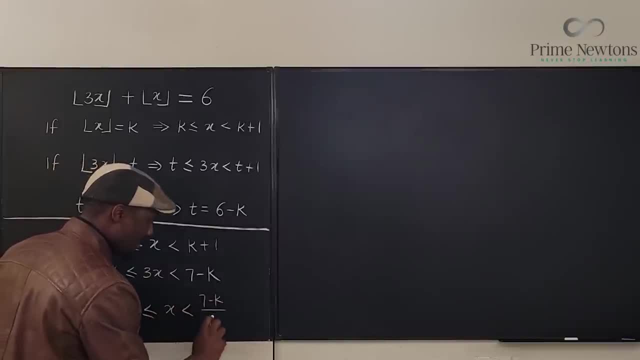 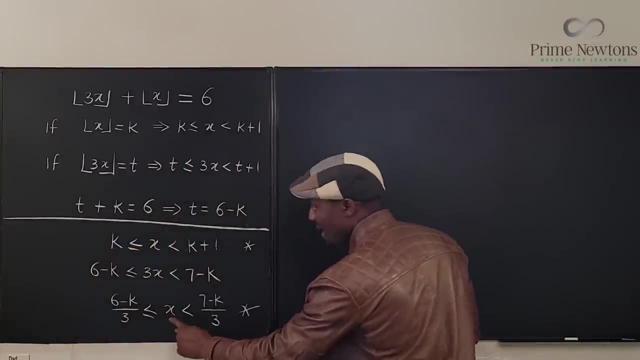 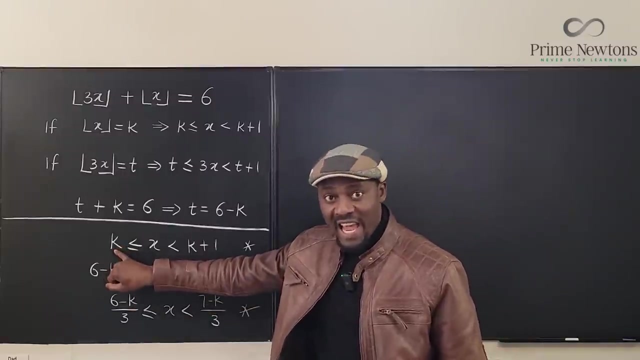 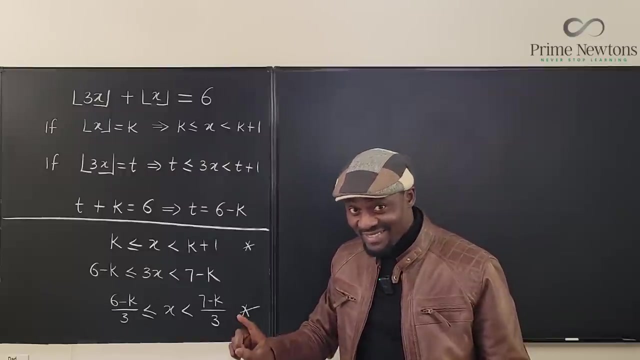 and it is less than seven minus K divided by three. So look at this and this. They both have X in the middle. So now let's do some comparison. We know that K is less than or equal to X, right, Nice? 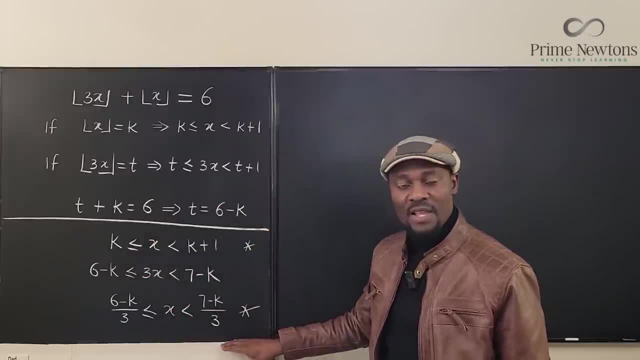 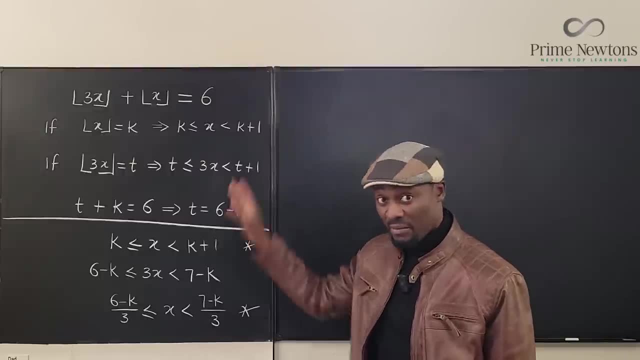 Now from here, let's just jump to this side. We know that X is less than seven minus K over three. This is certain. We got that from all the definitions we've used. So definitely, because K can never be less than or equal to X. 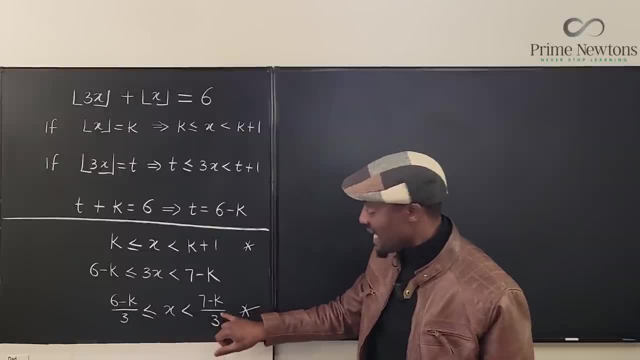 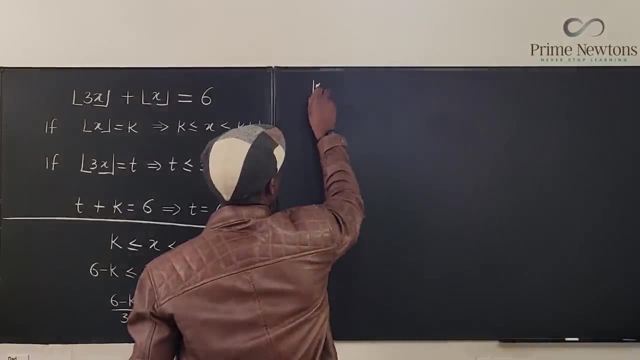 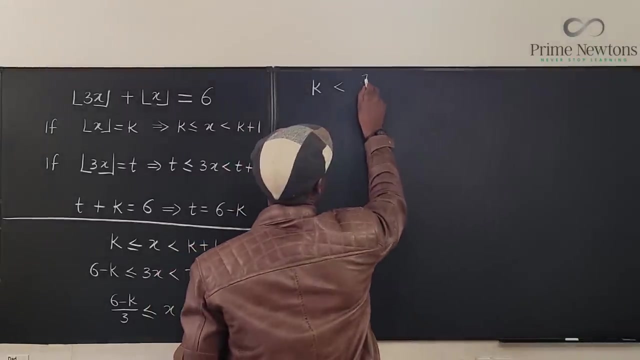 it cannot be more than X, And we're sure that X is less than this. We know that K is less than this, So we can go here and say K is clearly less than no option of equal to seven minus K over three. 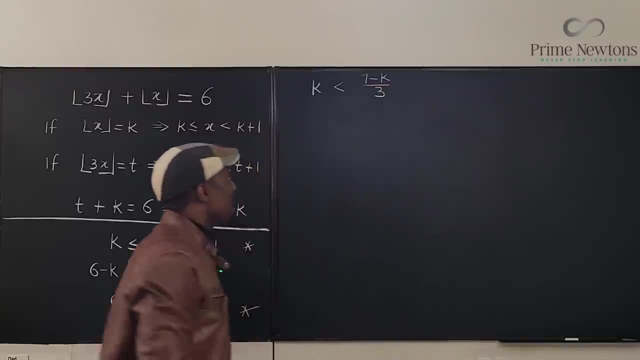 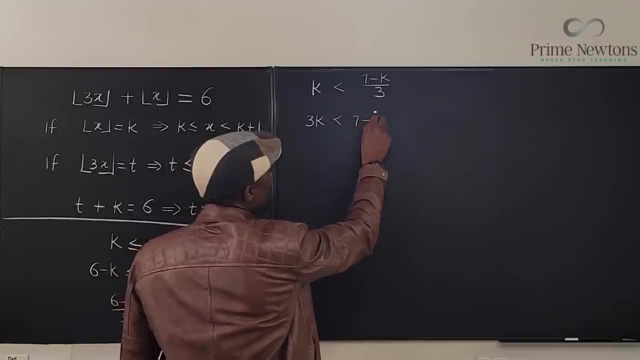 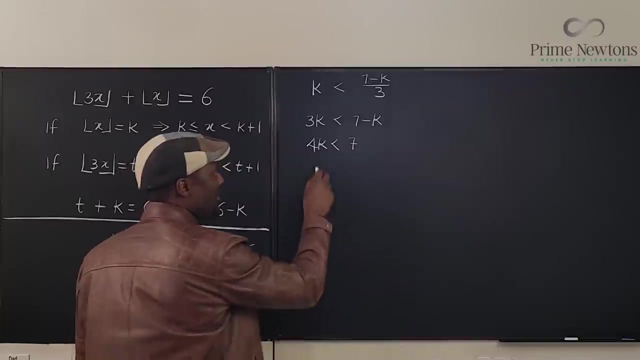 seven minus K over three, And then we can solve this inequality. We get three: K is less than seven minus K. Let's pull one K over here. We have four. K is less than seven. What do we have? We have: K is less than seven over four. 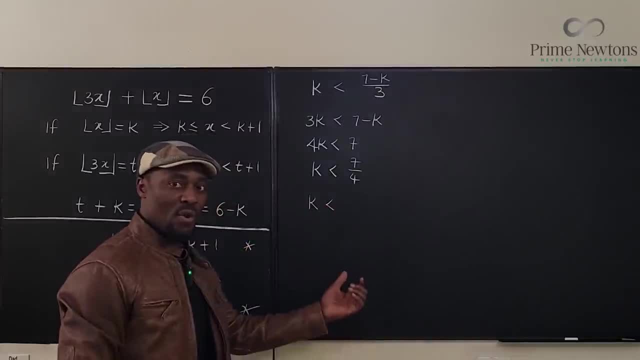 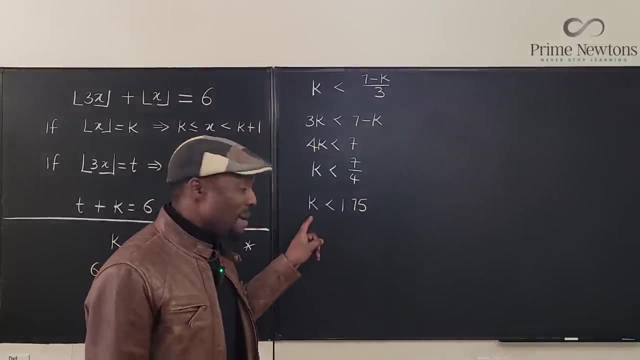 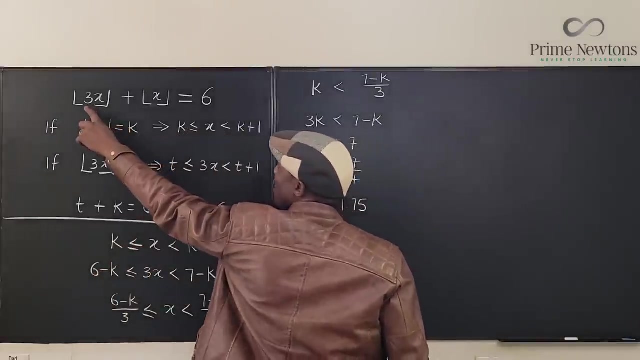 So K is less than 1.75, right, So we can call it 1.75.. Okay, Well, remember, K is an integer, right, And it's a positive integer because, look, we're adding the floor of a number plus something gives you. 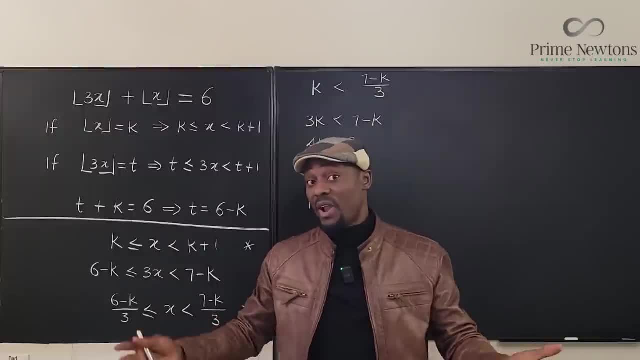 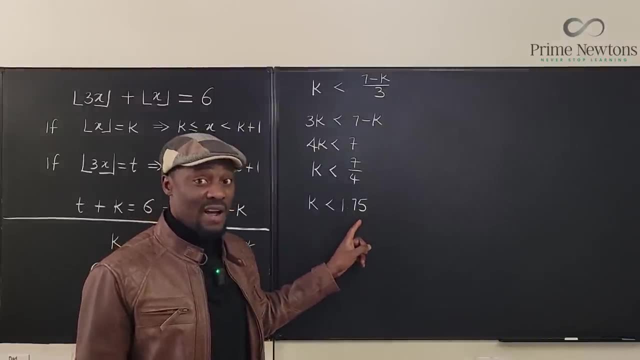 a positive number means that the things you're adding are positive. There's no subtraction anywhere. So we know that if K is a positive integer and it is less than 1.75, it has to be one. That's the integer, the only integer that is less than 1.75.. 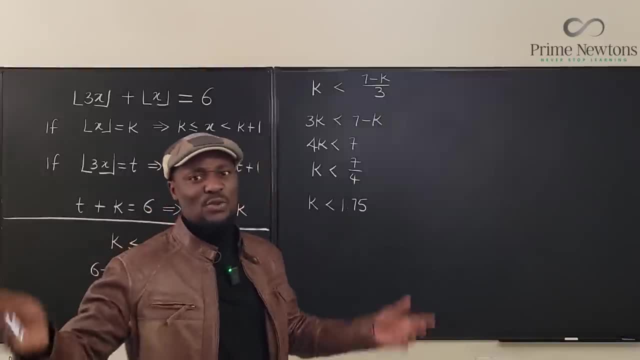 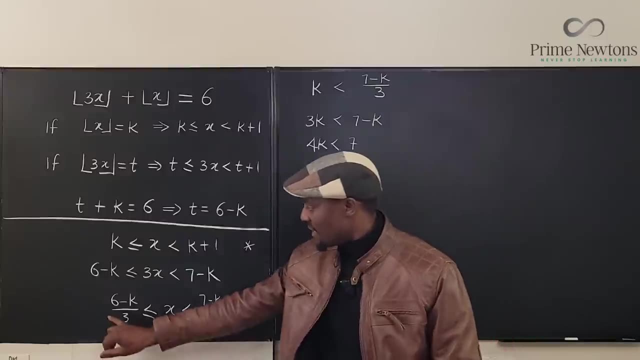 Hey, this is not X. We're still talking about K, but let's assume. we're not sure what it's gonna be. Let's just wait, We're gonna go back to it. So let's go again. We're gonna go to this side. 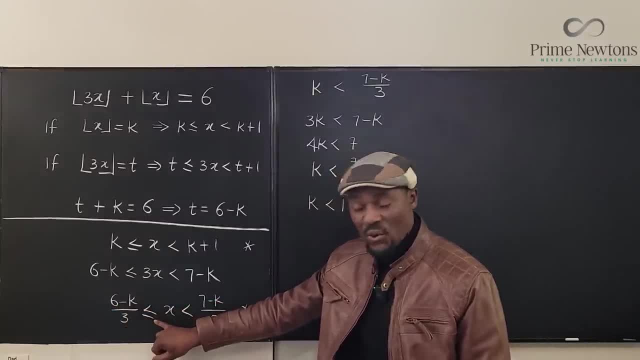 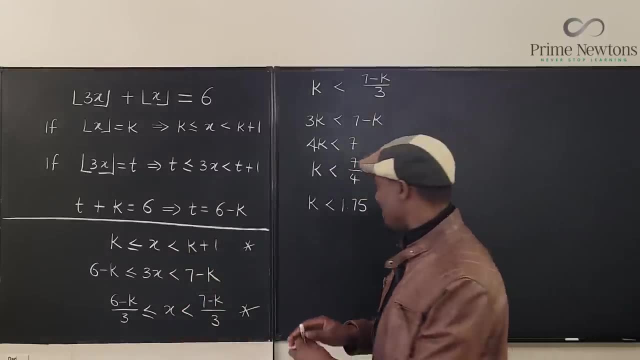 We know that six minus K over three is less than or equal to X. But here we know that X is less than K plus one. We can do the same thing we just did here. Let's do the same thing, Okay. We know that K is less than 1.75.. 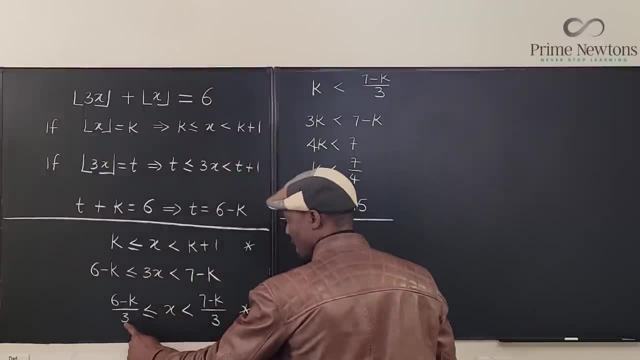 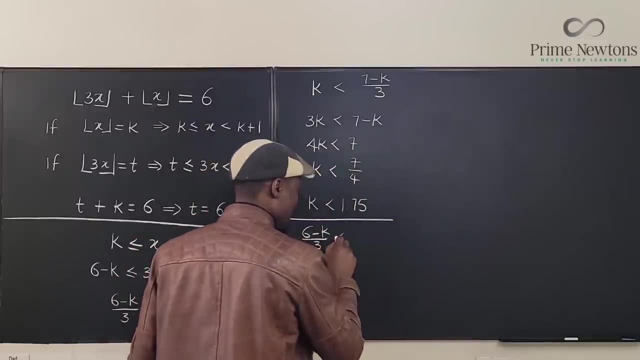 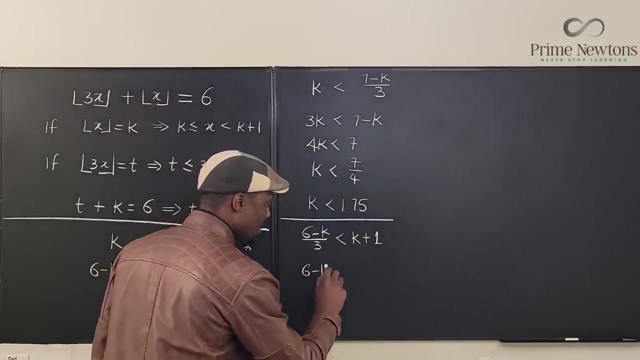 We also. let's do the same thing. Six minus K over three is less than K plus one. So if we multiply both sides by three, we're gonna end up with six minus K is less than three. K plus three Negative four K. 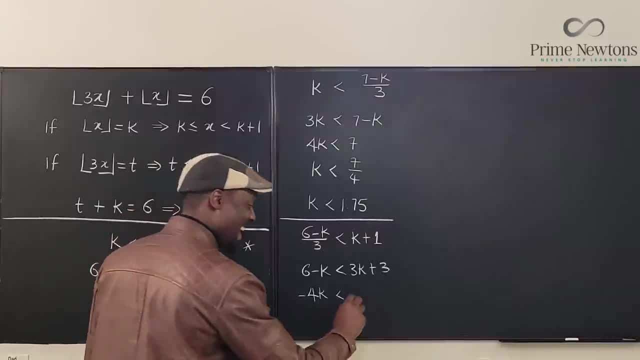 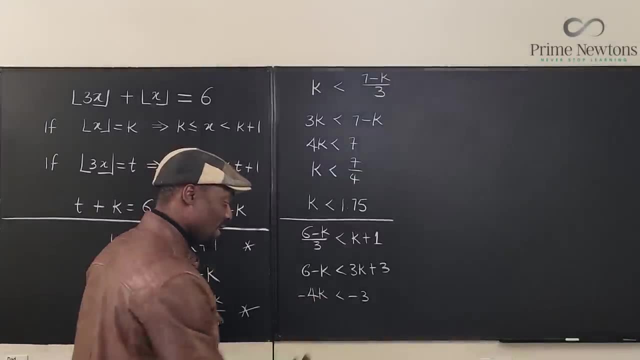 Oh, negative four, K and this is gonna become- I got scared- negative three. So what we have is, if you divide both sides by divide both sides by negative four, the sign is gonna change to a greater than, and then you have K will be equal to three over four. 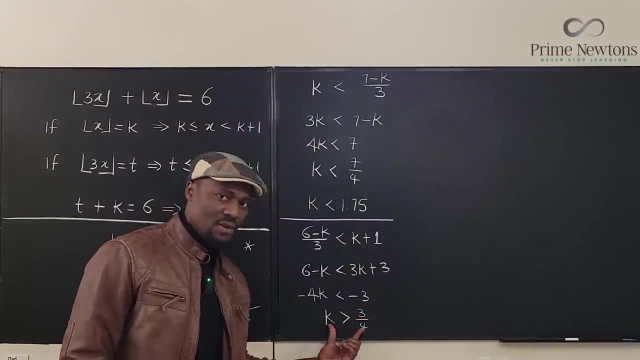 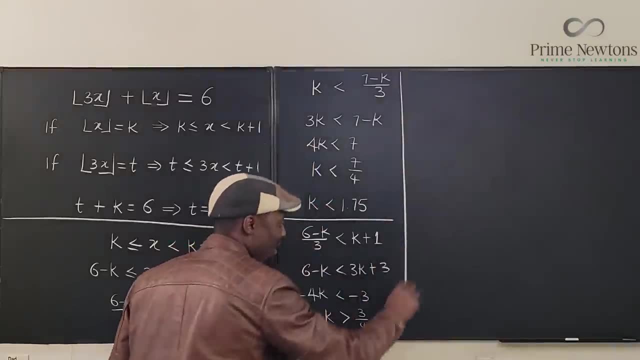 I mean greater than three over four. So K is greater than three over four and K is less than seven over four. Oh, it's beginning to look juicy. Let's look here. What do we have? So we have: three over four is less than K. 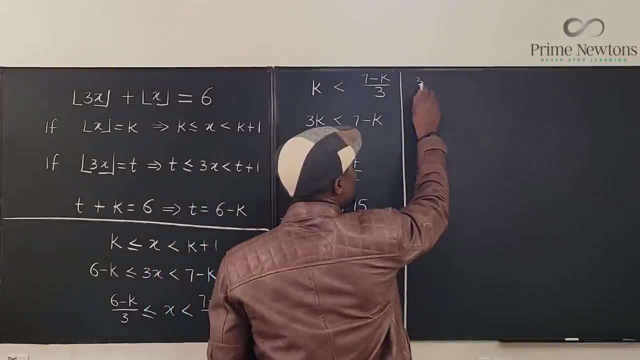 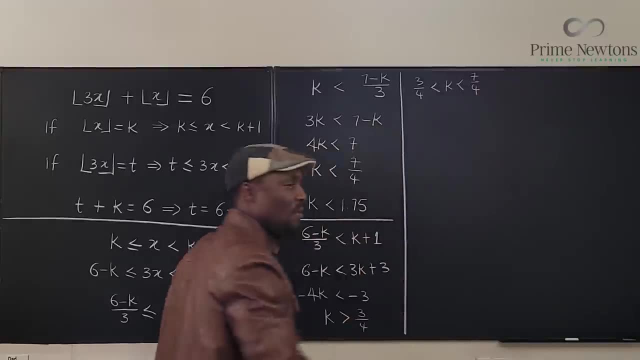 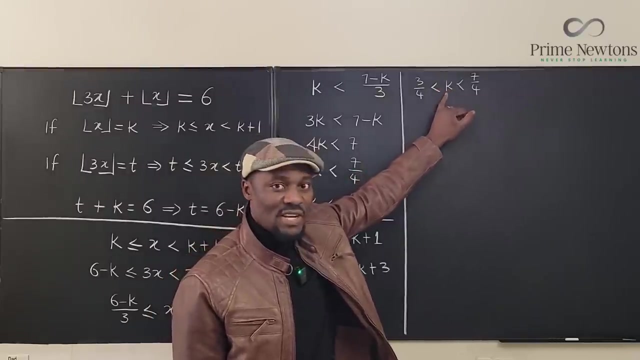 but K is less than seven over four. So it's like this: Three over four is less than K and K is less than seven over four. See what we have. This is 0.75.. It's less than this integer, And this integer is less than seven over four. 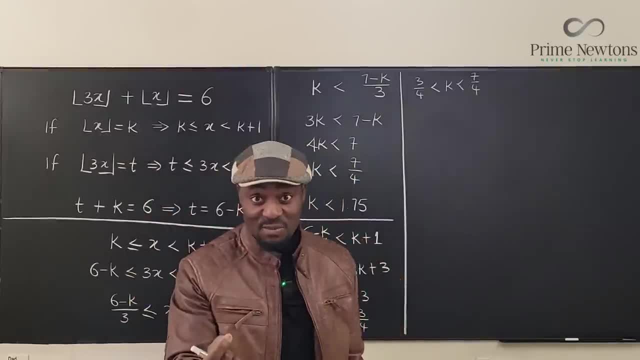 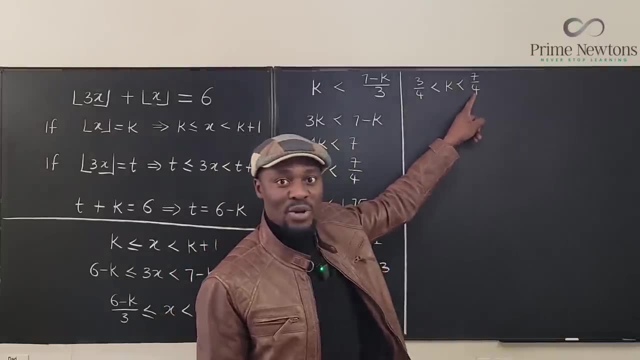 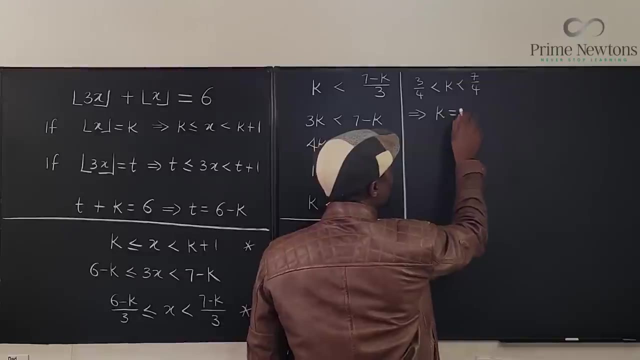 See, I could have told you that, because it's all positive, Our K is supposed to be one, but now we can prove it. The only integer between a proper fraction and 1.75 is one. Okay, this implies that K is equal to one. 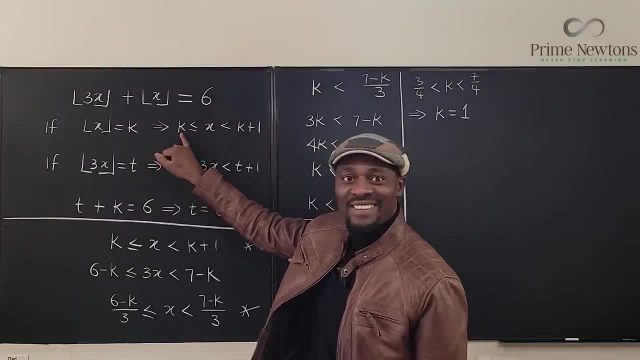 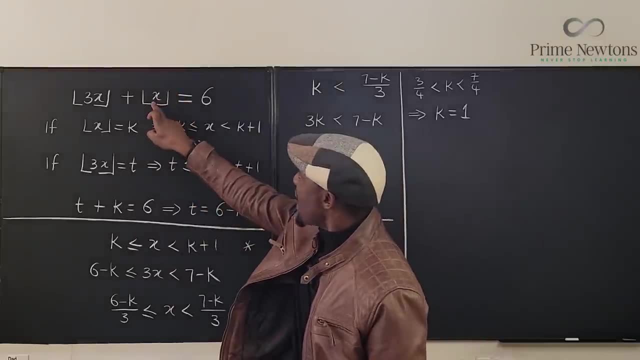 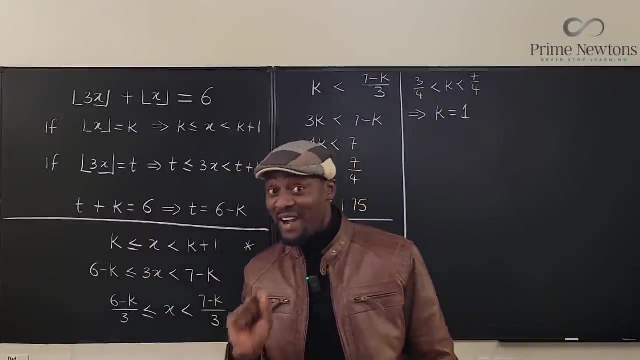 So we have found K. Now what does this mean? It means that the number we have here is one point, something We haven't found: X. Remember, we need to find X. So what we found now is the floor of this is one. 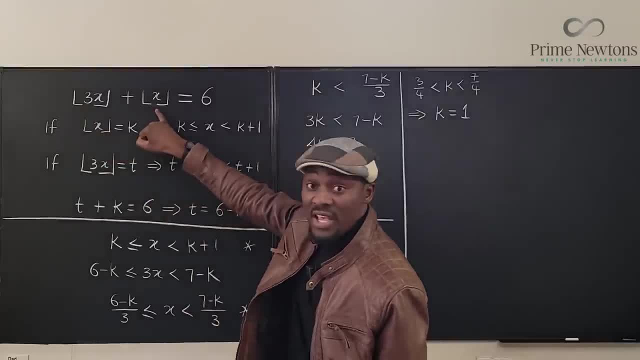 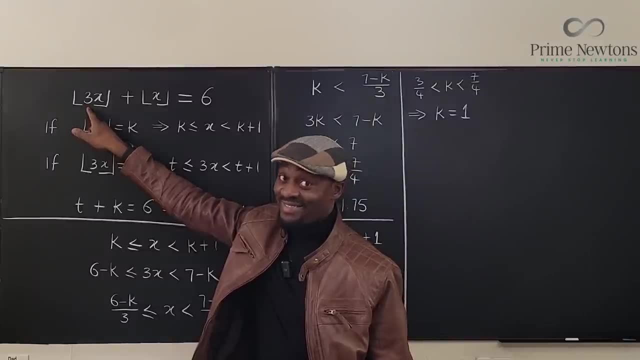 The floor of this? we don't know, But if this is one and if you add this to this, you're gonna get six. It means the floor of this is five. Right, you get it. So let's go back to all the conditions that we have. 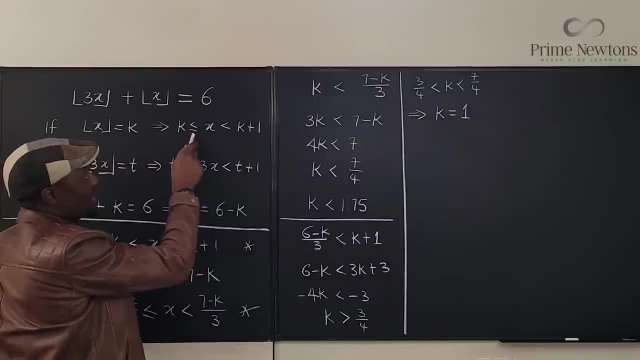 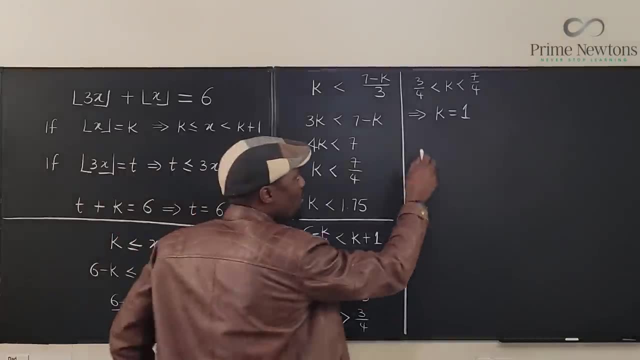 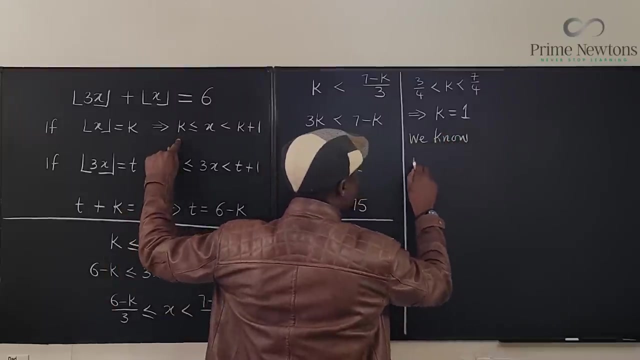 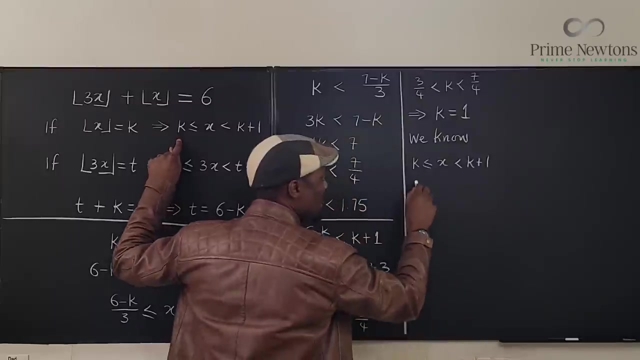 We know that one is less than or equal to X and X is less than two, So that's gonna be one plus one. So let's go again. So we know that K is less than or equal to X and X is less than K plus one, which means one is less than. 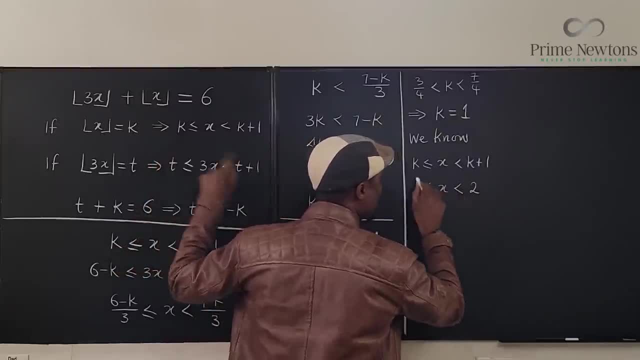 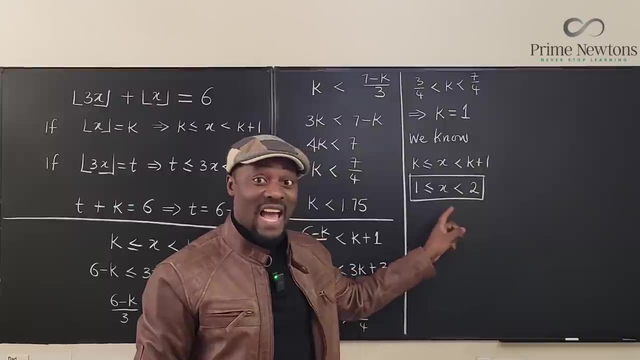 or equal to X, and X is less than two. This we know. Our answer is between one and two, But this is too wide a gap. We need to figure out exactly what would make this work. So let's go back to here. 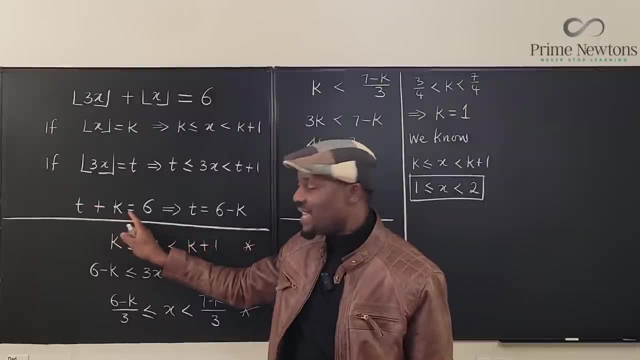 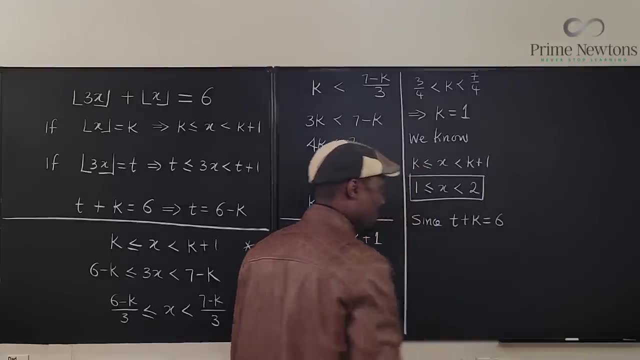 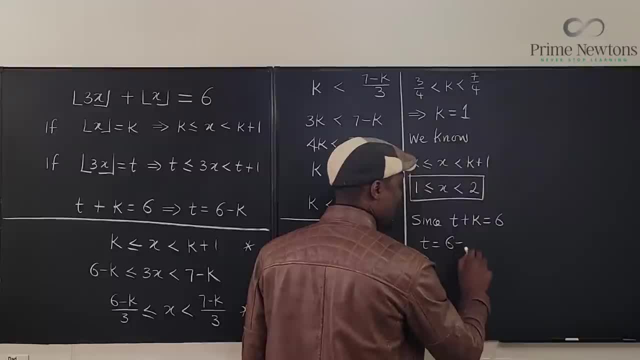 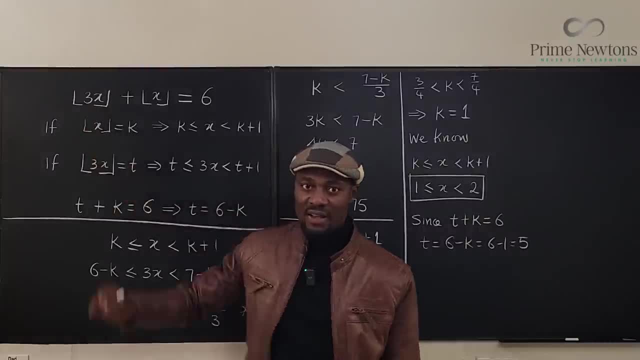 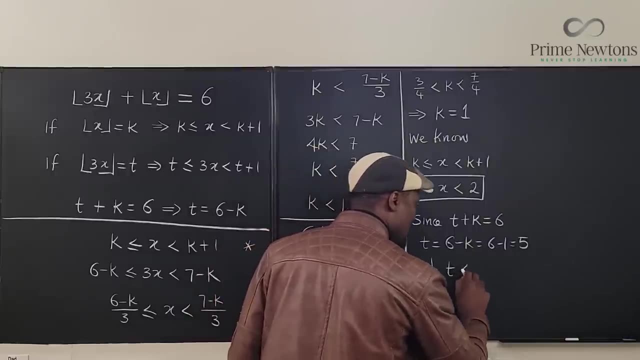 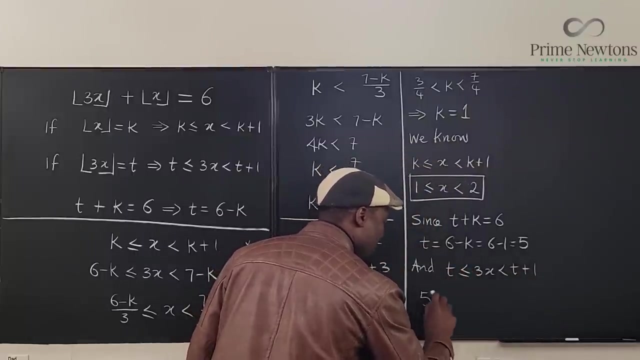 So the floor of this is five. So therefore we can say- and let's do it again- T is less than or equal to three X, less than or equal to T plus one. So we know that five is less than or equal to three X. 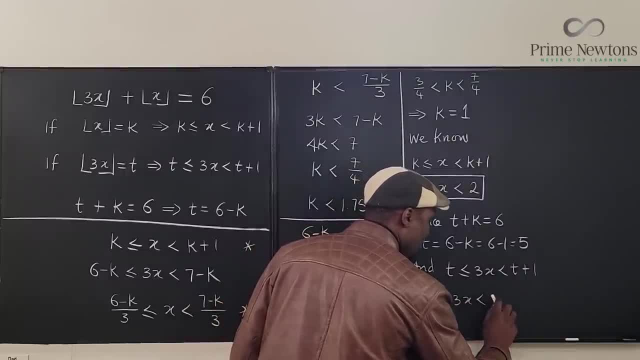 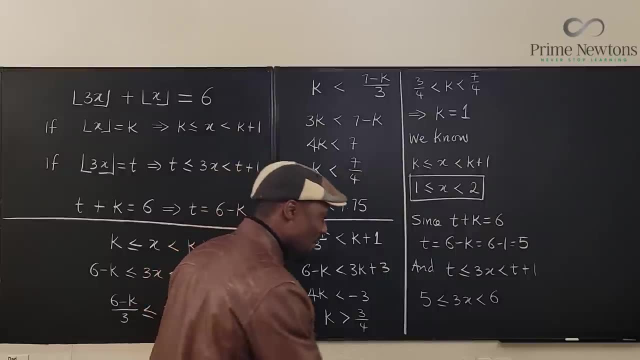 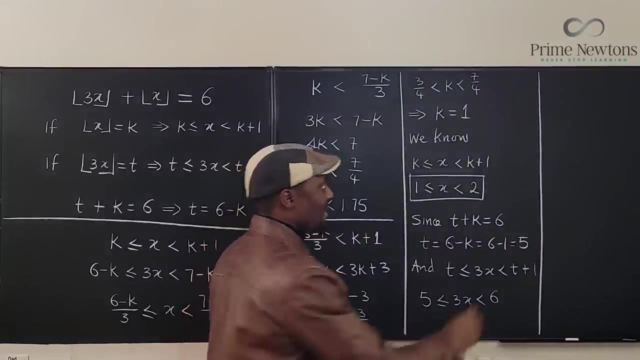 and this is less than or equal to three. X and this is less than six. five plus one. So what exactly is the value of X? Divide everything by three. you will notice that. let's do it here. You will notice that five divided by three.